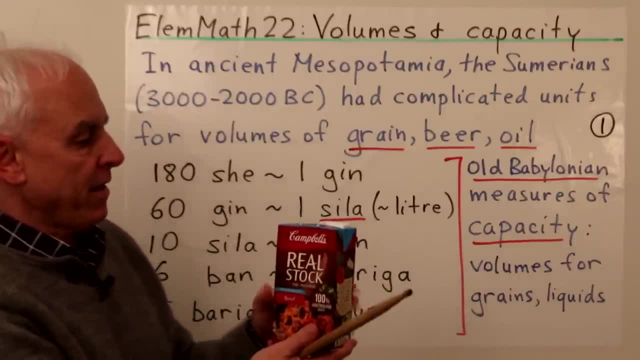 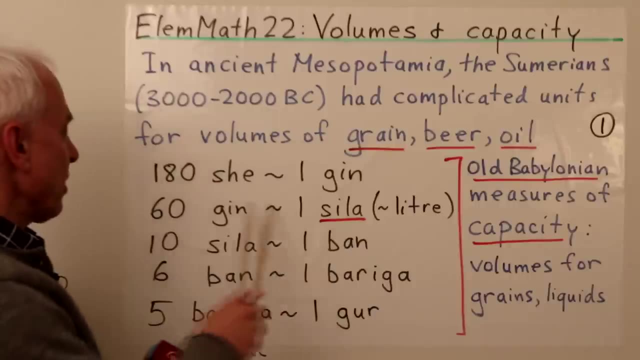 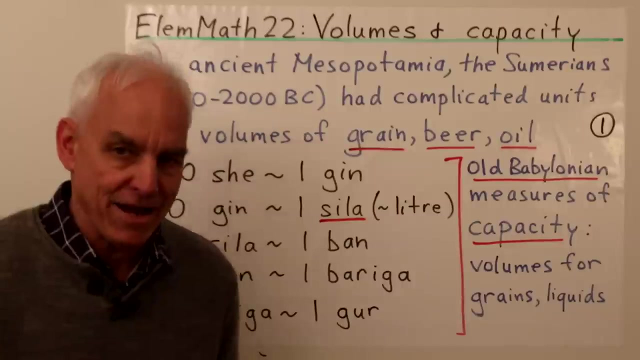 of volume and that's roughly comparable to what the old Babylonians called a silla. Now, the silla itself was composed of 60 gin, and one gin was composed of a much smaller unit, a shea. So 180 shea was one gin And, in terms of sillas, 10 of them formed one ban. six ban formed one bariga. 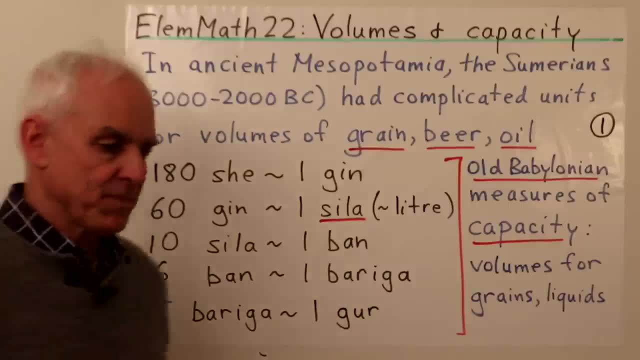 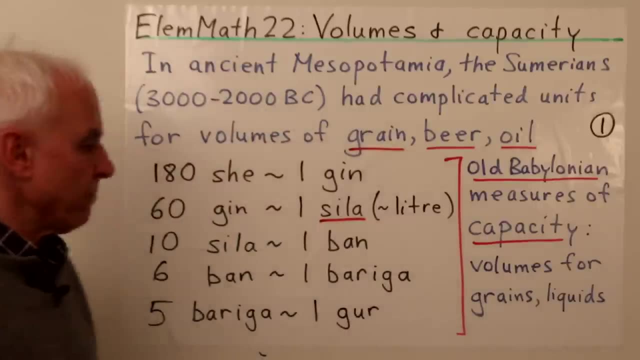 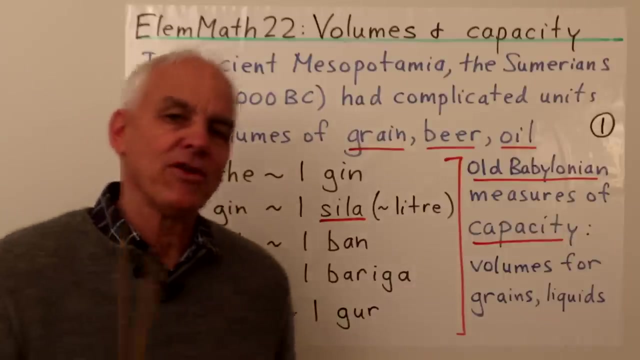 and five bariga formed one gur, So we definitely had these different units being able to measure different scales of quantity, Lots of things or perhaps very small ones. Now, while we sometimes use the word volume, sometimes it's maybe a little bit more instructive to use the word capacity. 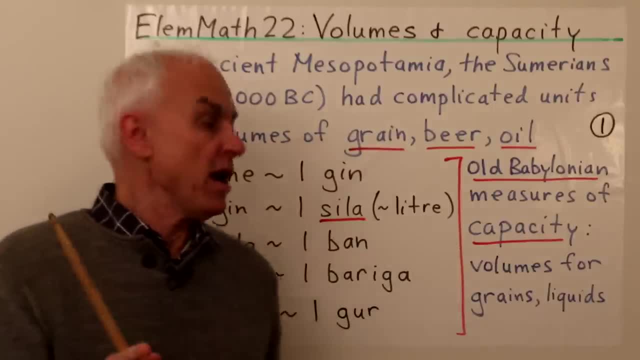 And capacity refers to volume in the context of grains or liquids, More so than, say, the volume of a box, Usually rather in terms of a liquid or a grain. So this is a topic that goes back to antiquity And it's a very important topic and a very instructive one for young children to 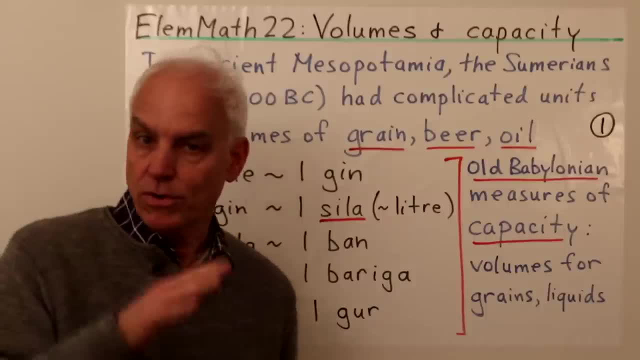 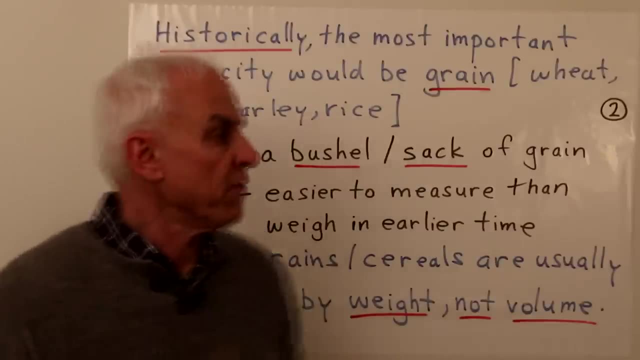 strengthen their arithmetical understanding and connect with the real world around them. Historically, the most important capacity would have been grain, because that was the primary food: Grain- perhaps wheat or oats or barley or rice, etc. So we might have something like a bushel or 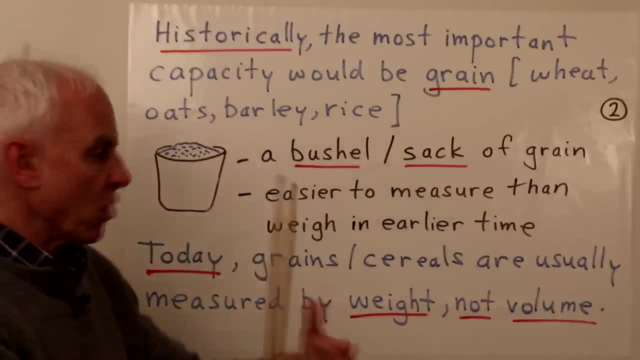 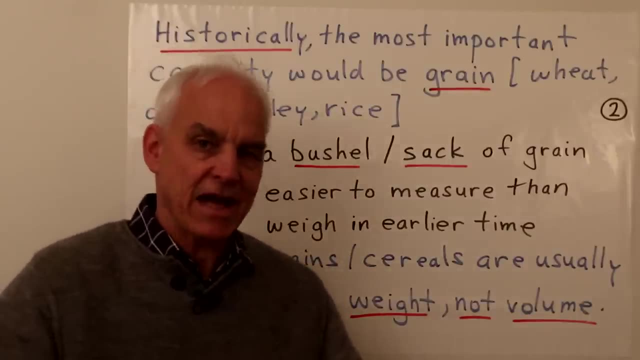 a sack of grain That represents a certain quantity, which was easier to measure than weighing it. So sometimes weighing especially heavy sacks of stuff was more problematic. These days, of course, weighing is actually easier because we have these scales and you can weigh things very easily. But back then, 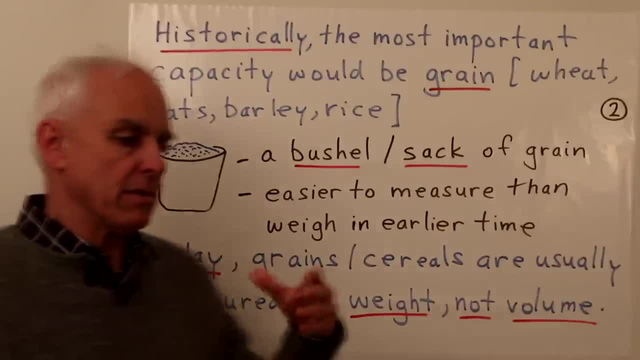 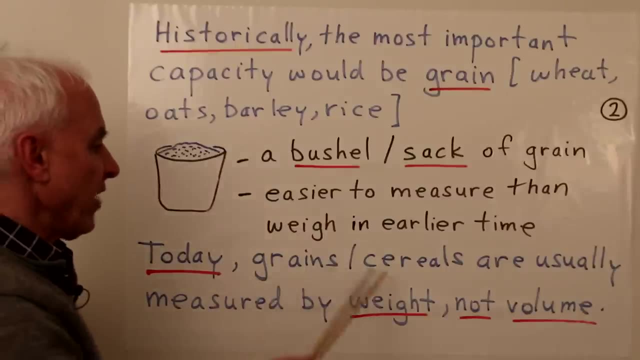 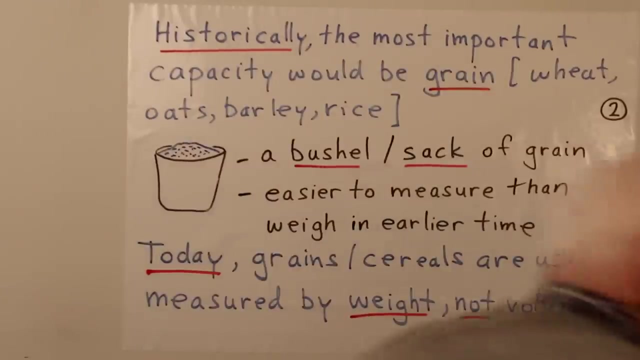 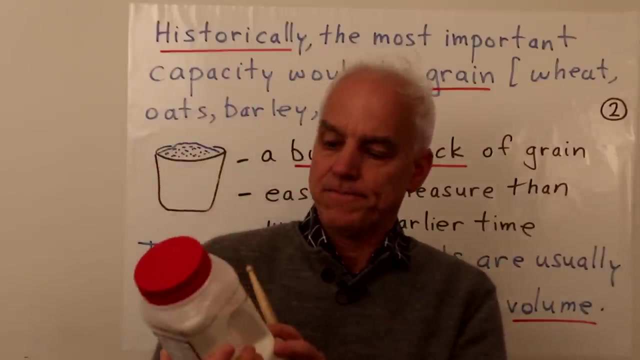 volume or capacity would have been perhaps more used for describing how much grain we have, While today, grains and cereals are usually measured by weight, not volume. So, for example, in our kitchen we have a tub of self-raising flour. So that's a grain And it's measured by. 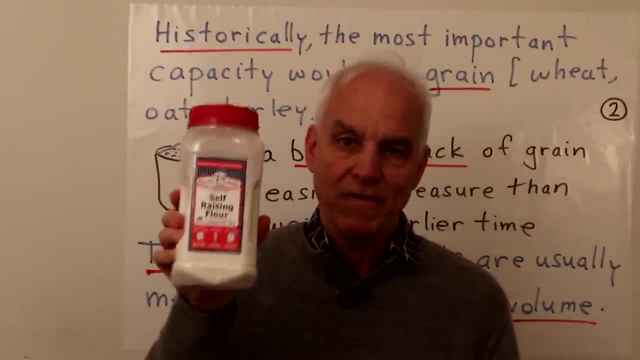 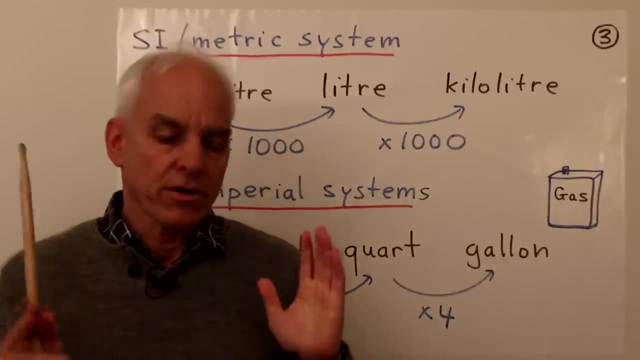 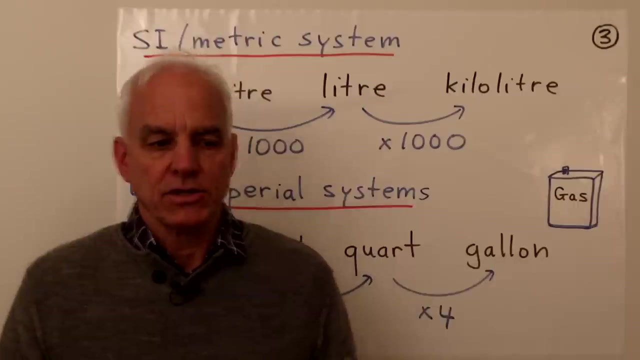 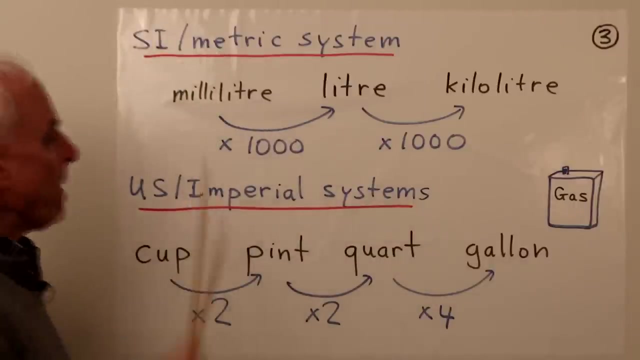 kilogram. This is one kilogram of flour. That's a weight unit, not a volume or capacity unit. Now, the modern system for measuring capacity or volumes is a little bit complicated, And so here we'll remove it, and we'll leave some additional complexity for a later time In the SI or the 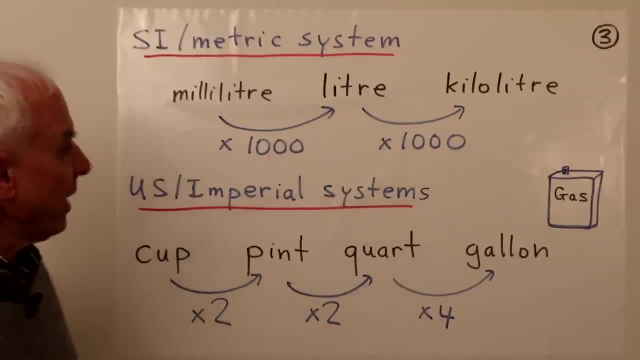 metric system. the basic unit, we've already said, is the liter And in terms of liters, a thousand of them is a kiloliter And the subunit of a liter is a milliliter, which is one thousandth of a liter. So a thousand milliliters is a liter and a thousand liters is a kiloliter. So again we see the 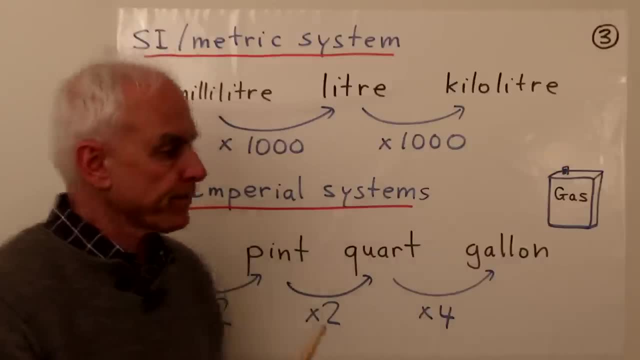 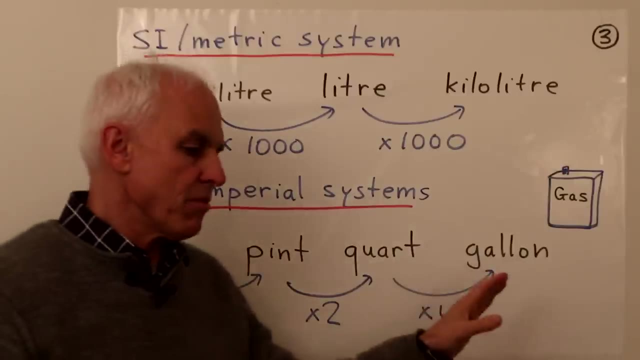 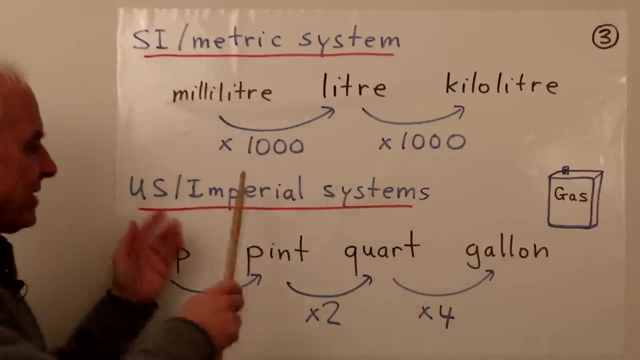 difference going from one unit to another unit. Now there's a second system, the US or the Imperial systems, which have more or less the same structure, but the units are actually a little bit different. So there's actually two separate systems here, although they're very closely aligned, And there 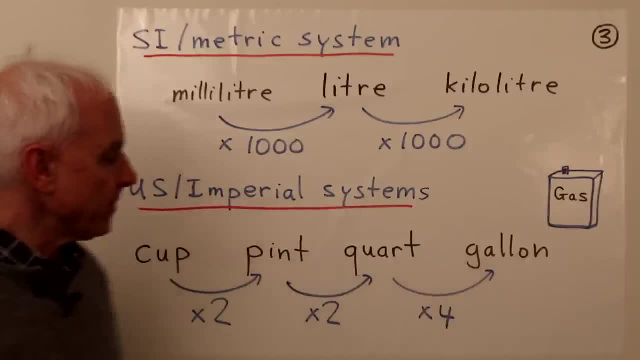 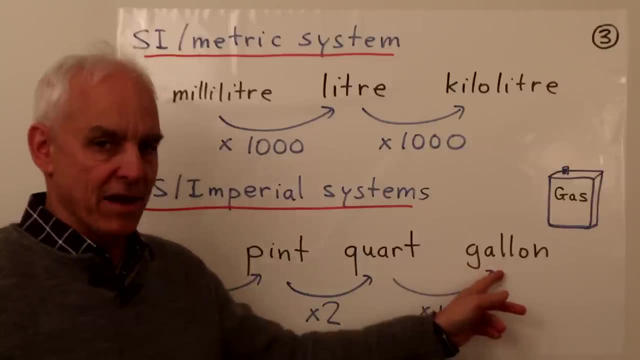 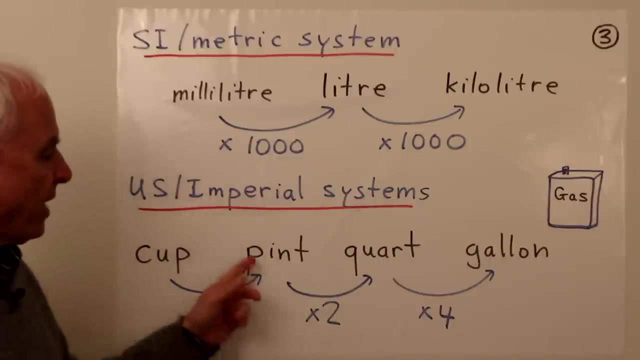 the units are the cup, pint, quart and gallon. So if we think of the gallon as being sort of the fundamental unit, then the quart is a quarter of the gallon, Hence the usage word quart. So four quarts to a gallon And then a pint. well, that's half of a quart, or two pints make a quart. 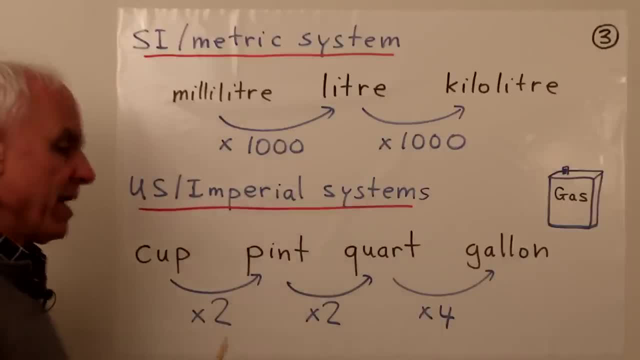 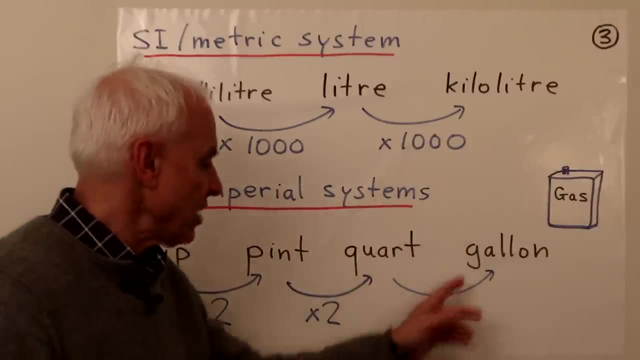 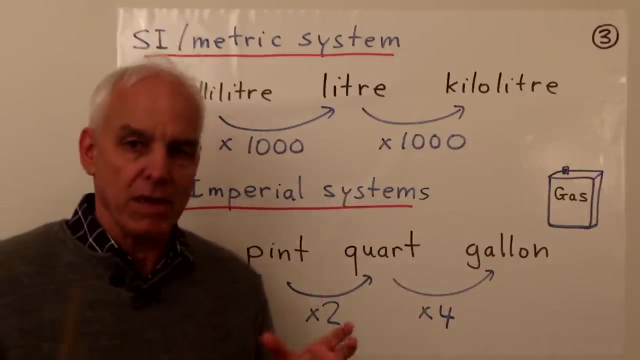 And a cup is half of a pint, So two cups make a pint. So this is a very sort of human-based system. These ratios are quite small and easy to work with, So these are actually quite convenient for, you know, drinking beer and consuming liquids and so 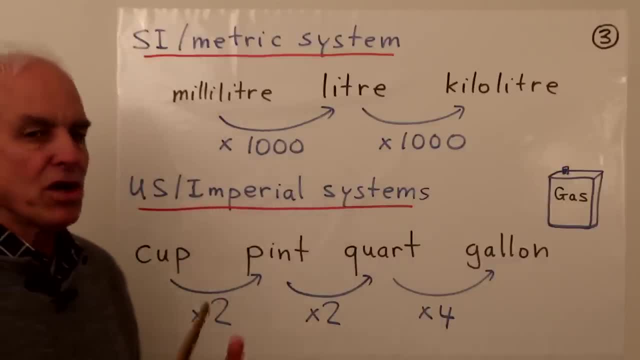 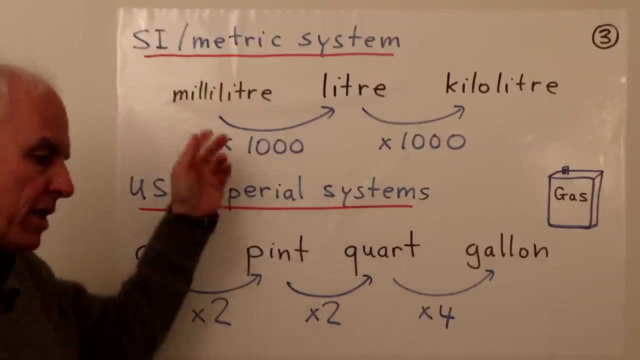 on and making making kitchen recipe kind of computations. This system is the more scientific one. It's more precise, We have a greater subdivision, But on the other hand the numbers involved are typically larger. So in Australia of course we use the metric system So we can look in. 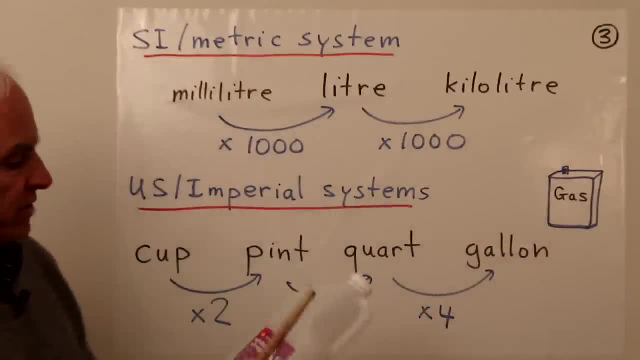 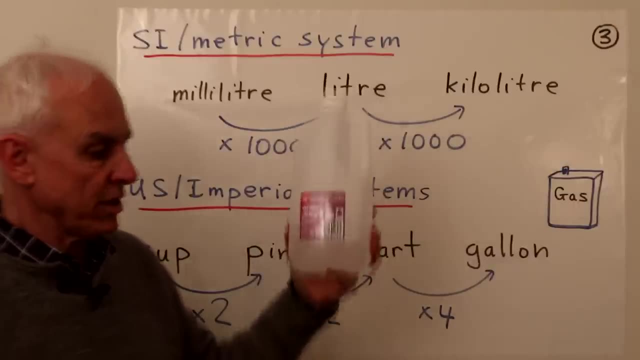 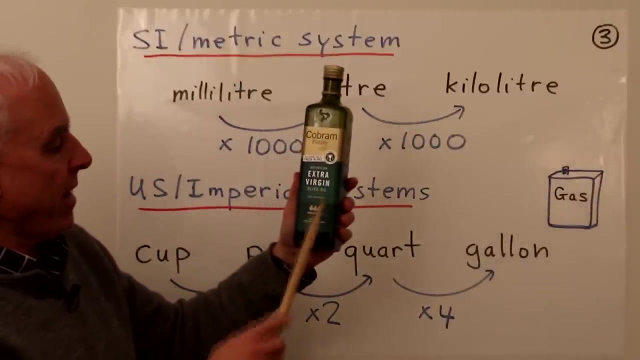 our fridge and we can find various. So, for example, here is a bottle of vinegar, white vinegar, and two liter bottle, So there's a two liter bottle. Here is some extra virgin olive oil and we see that it's 750 milliliters. Okay, so ML. 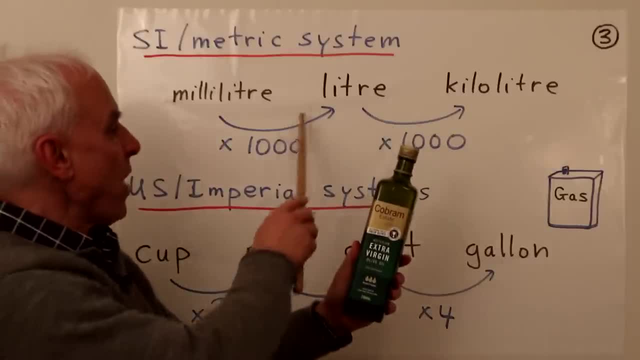 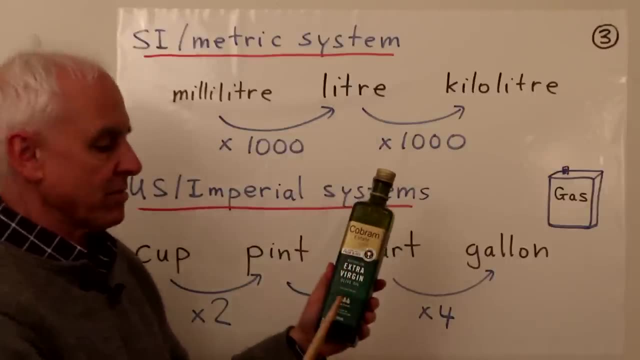 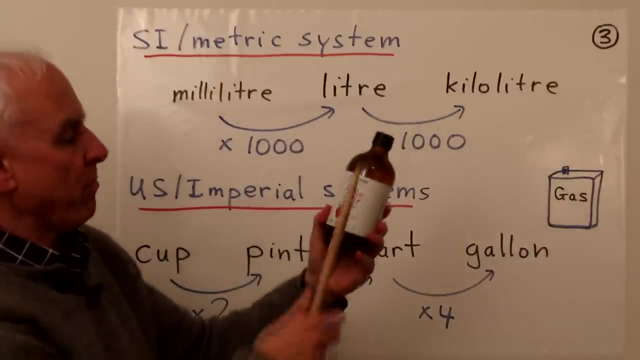 is a short form for a milliliter, So 750 is not quite a thousand. That's going to be some fraction or some portion of a liter, Not quite a liter, but not too far away from a liter. also, What else do we have here to show you? Okay, so here's some apple cider vinegar And down here. 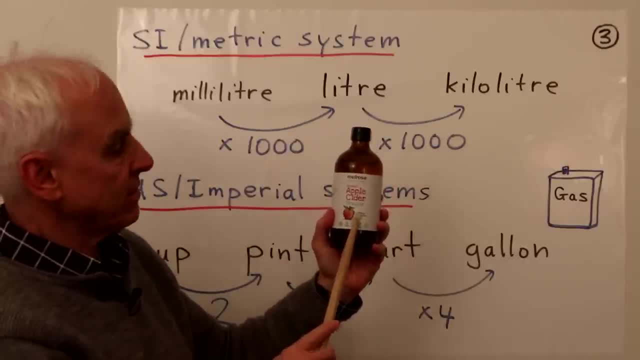 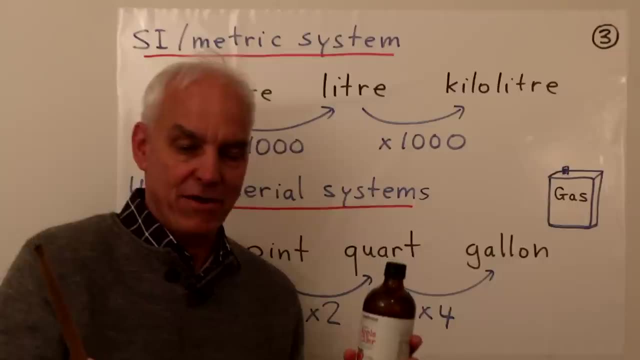 you will not be able to see, but it says 500 milliliters, 500 milliliters. Well, 500 is exactly half of a thousand, Or 500 plus a 500 is a thousand. So this is one half of a liter, Two of. 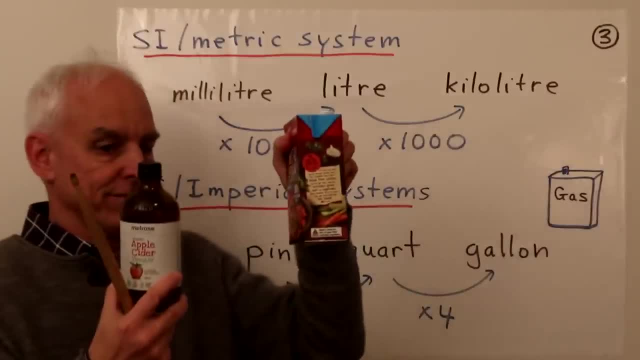 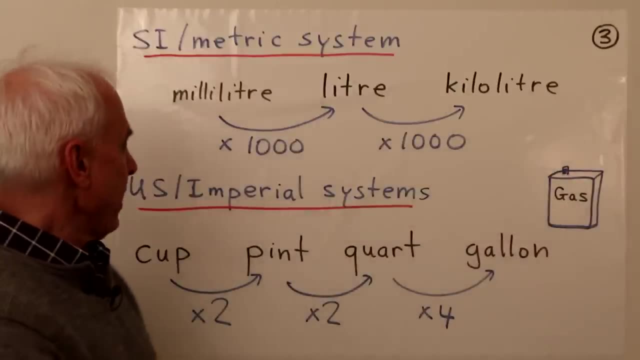 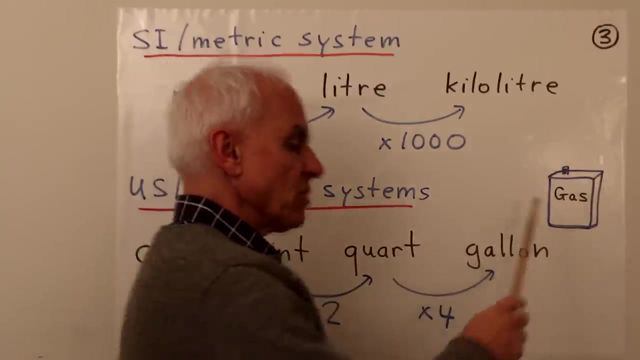 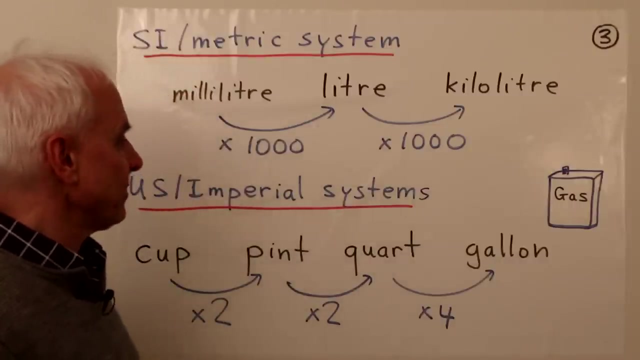 these would make one liter Okay, and maybe we should say the gallon. in the US imperial system is often associated with gas. That's sort of how much a standard portable gas canister has in it. So these are the the two systems that we conveniently use. But there is a little bit. 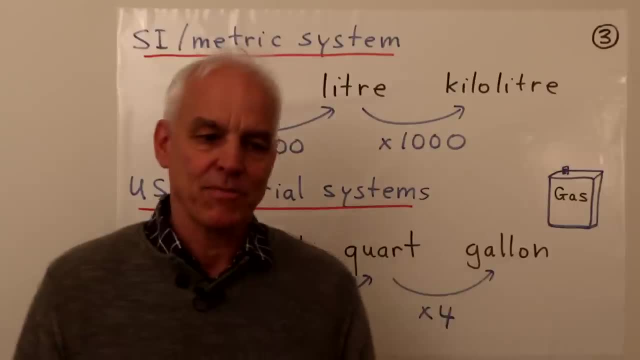 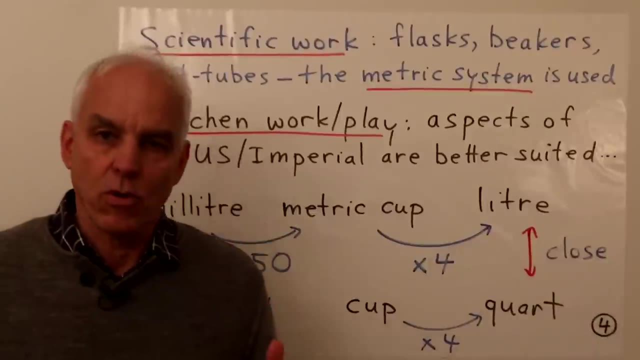 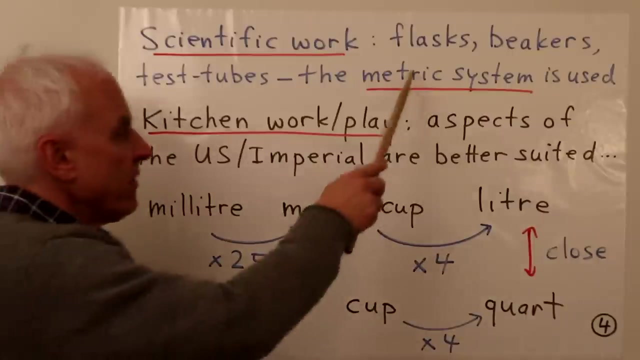 of overlap and there's some extra complexity that we should also talk about at some future point. It's not quite as simple as this. Now, for our scientific work around the world, the metric system is almost exclusively used, So any kind of scientific equipment involving flasks or beakers- 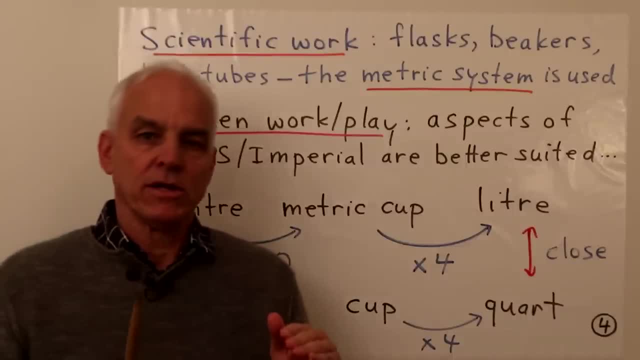 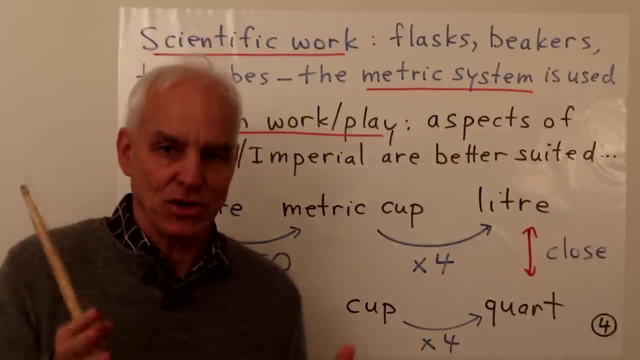 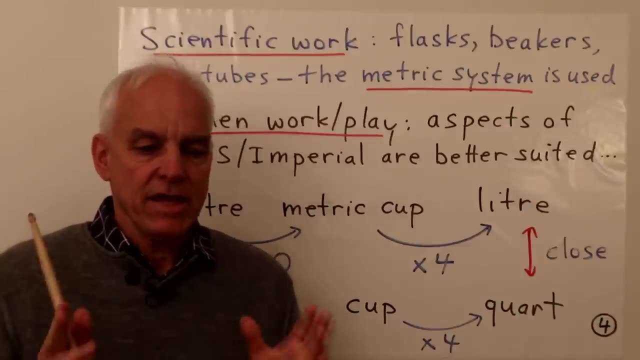 the kitchen, which is a very important application of volumes and in fact also weights, cooking recipes, baking cakes, etc. These things are often sometimes better served by the somewhat larger and more manageable units in the US or the imperial system, And so there's actually a little bit of a 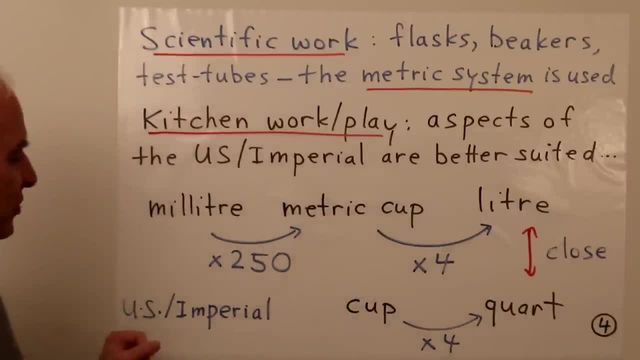 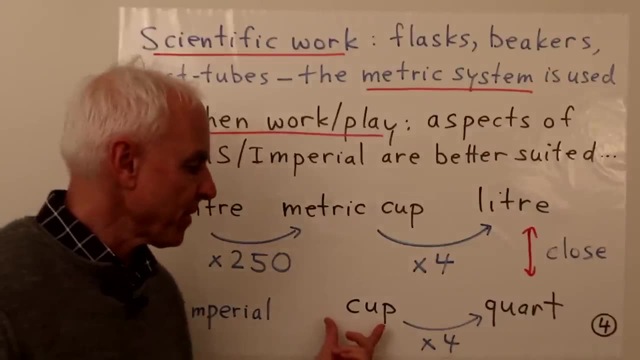 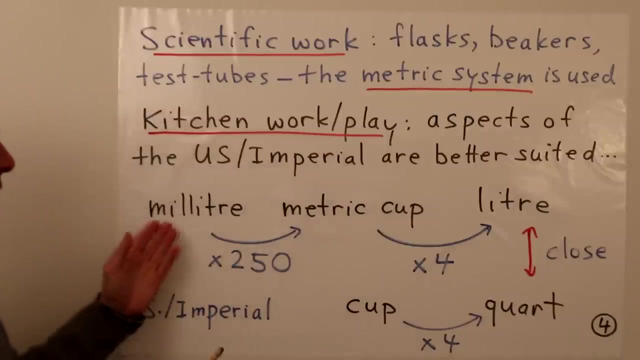 crossover. So I remind you that in the US or imperial system a quart consisted of four cups. So a cup times four is a quart, And that's quite a convenient kind of ratio of volumes and it's also sort of been adopted by the metric system also, Maybe not quite officially, but sort of 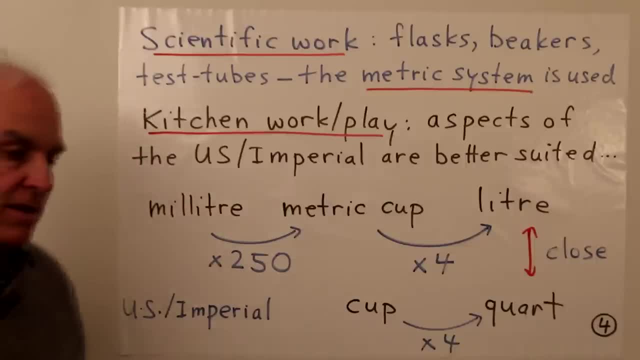 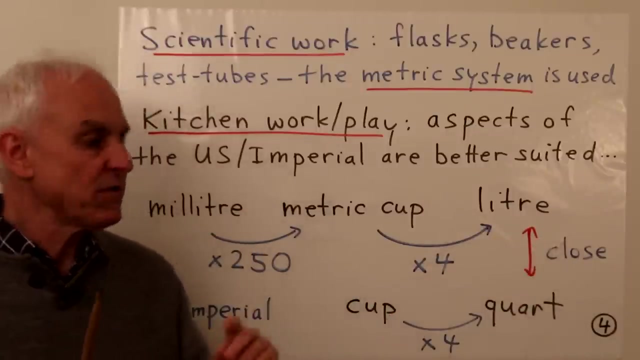 unofficially, especially when having to do with kitchen homewares. Okay, so we already talked about a milliliter and a liter. We know that a thousand milliliters is a liter. That means that a milliliter is a lot smaller than a liter, So it's useful to introduce a metric. 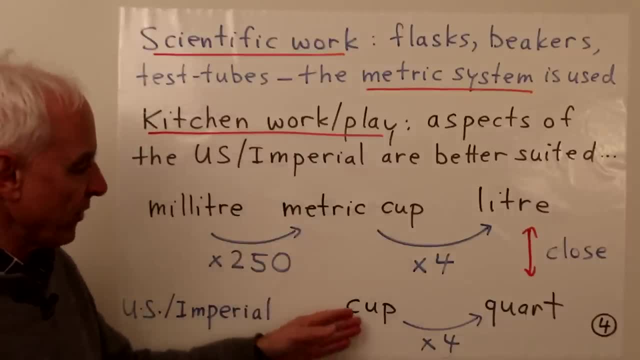 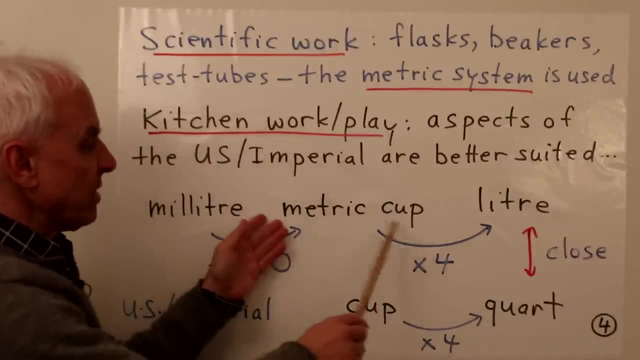 cup, which is playing the same kind of role as a cup in the US or imperial system. In this system, four of these cups equals one quart. In the metric system we say that a metric cup is a quarter of a liter, or four of these will make up a liter. 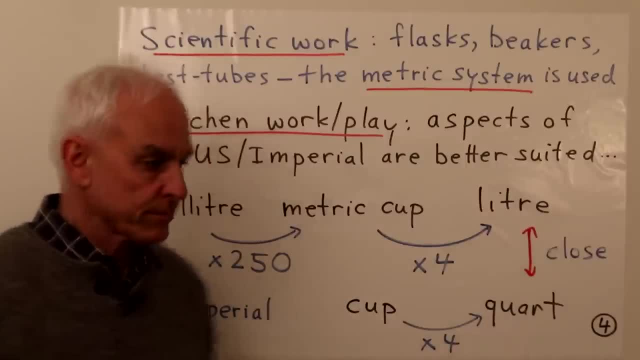 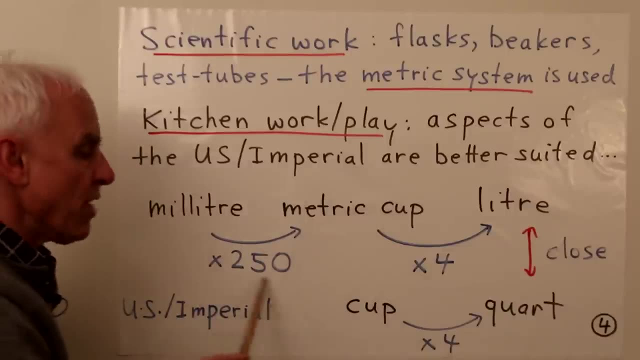 Just like four cups make up a quart, Well then it follows that in fact a metric cup consists of two hundred and fifty milliliters, because two hundred fifty times four is the thousand. So what we're doing is we're kind of appropriating some kind of units in the US or imperial system. 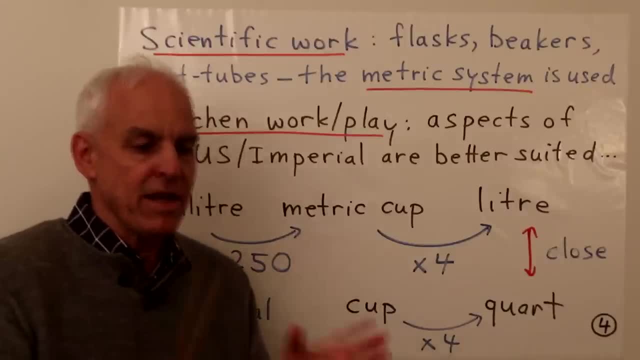 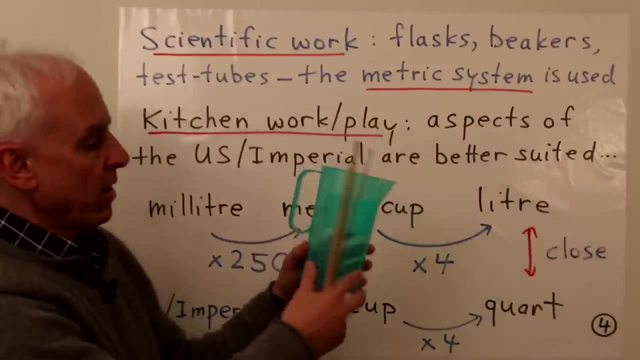 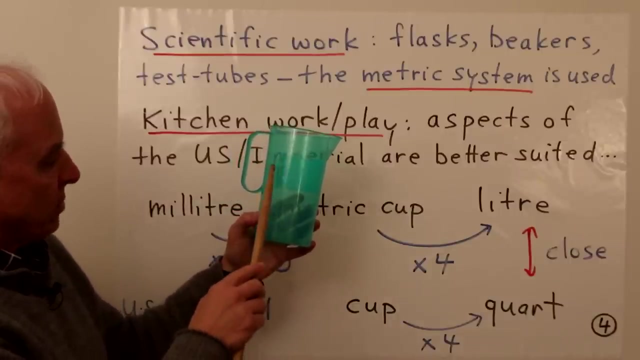 in the scientific or metric system, especially useful when we're working in the kitchen- world kitchen. So, for example, here is a beaker with some indications which you're probably not going to be able to see. There's one liter here, but in terms of grams. 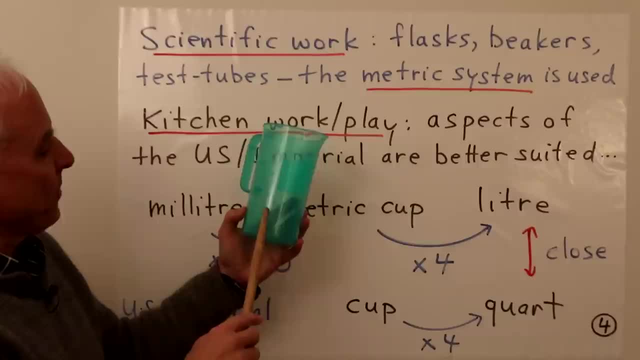 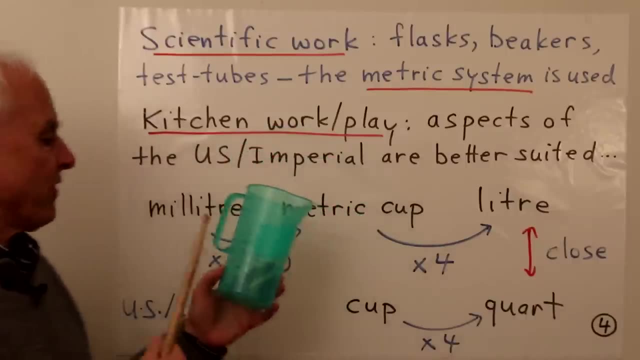 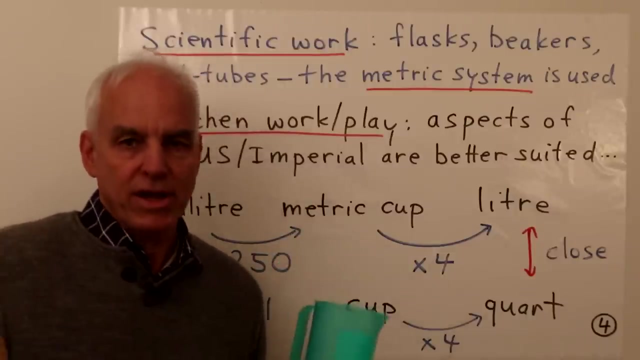 is also 750,, 500,, 250, but also, you can see that's one cup, two cups, three cups, four cups. So the notion of a cup is a useful additional tool, especially useful for metrical work in the kitchen when you're cooking or baking, So just as when 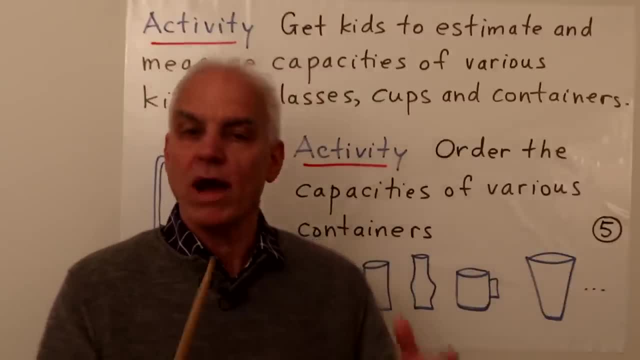 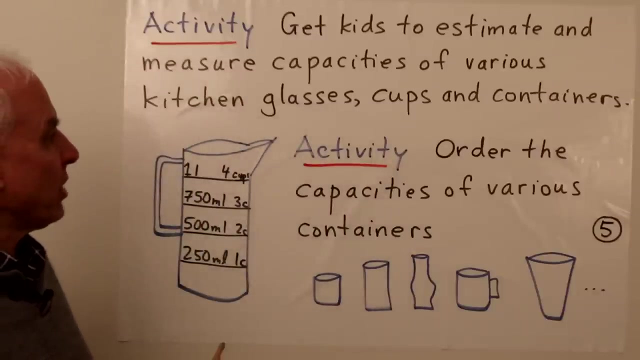 we were studying weights. we would like to encourage young people to go out and actually measure and record the volumes or capacities of various things that they find around the house or various amounts of fluid. So, for example, what we could do is get kids to estimate and measure the capacities of various 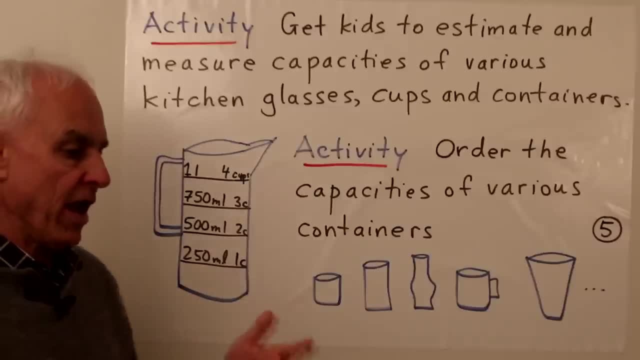 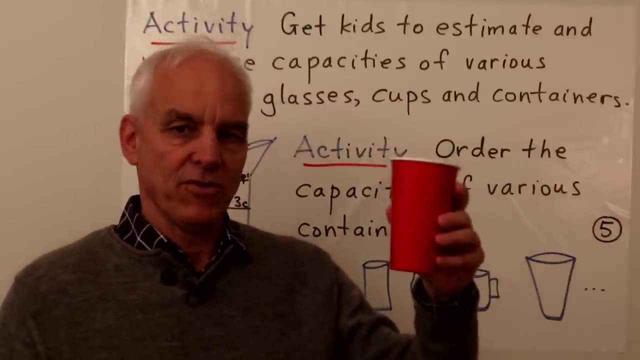 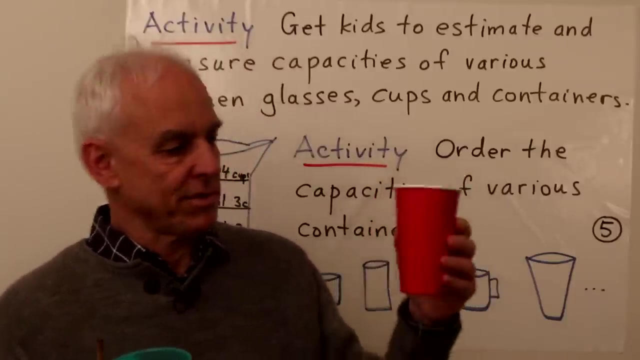 kitchens and kitchens, Glasses, cups and containers. So here is a plastic, paper cup and we could fill this with liquid and say: you know how much liquid is contained in this cup? Well, so the child could estimate what they think might be the volume, and then we can pour. 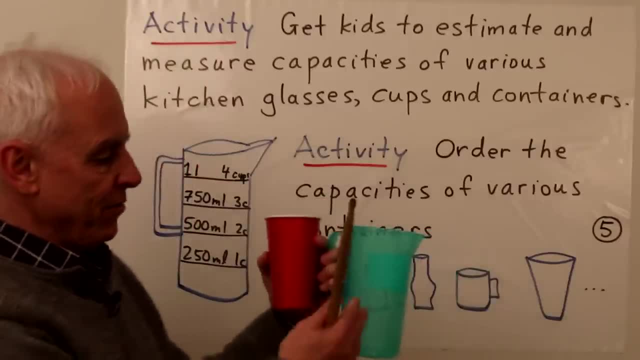 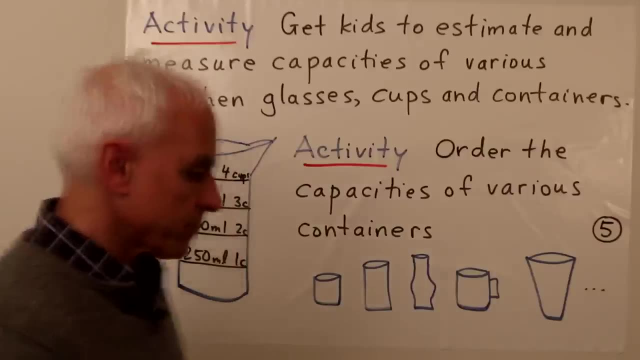 it into here and read off the level, and then we have a record of how much the capacity of the cup is. All right, We can do that, You can do this for a wide variety of things, And so with a little bit of experience then we could take a bunch of different. 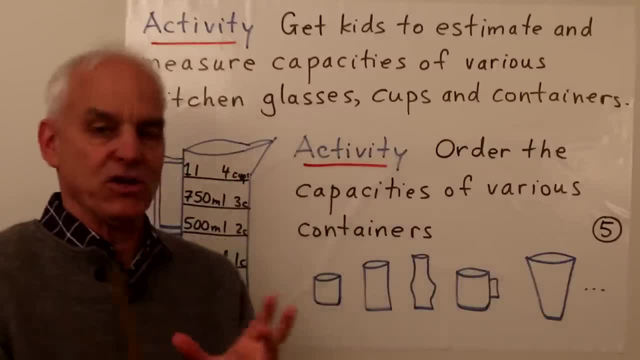 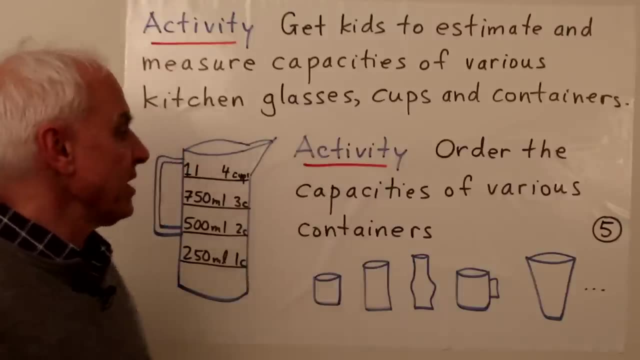 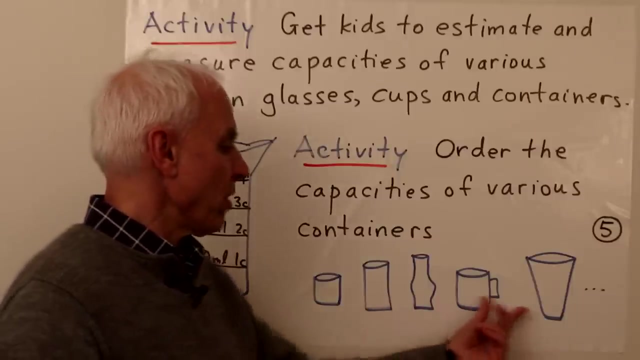 containers and kitchens are usually full of all kinds of different shape: glasses, containers, vases, etc. We can then, for example, order the capacities of various containers, Say starting with the smallest volume and then working our way up more and more volumes- In this case here- in order to determine which of these. 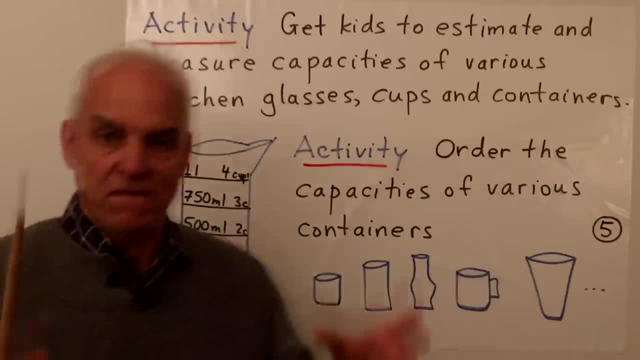 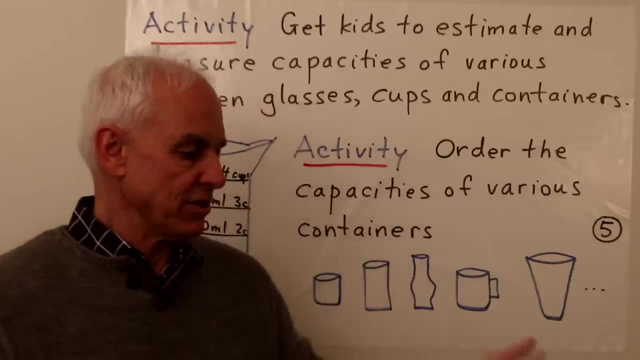 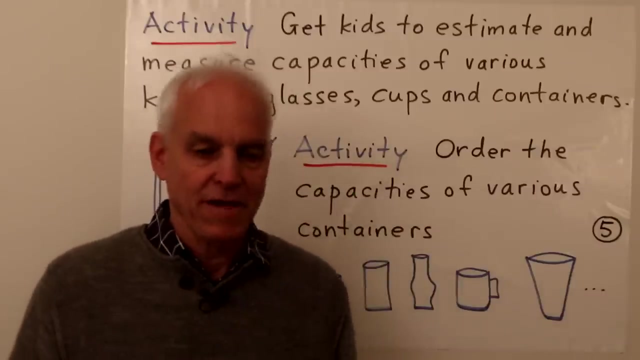 two say, has the greatest capacity. we would actually fill them with some liquid, presumably water, and then pour those quantities into a container and read the corresponding levels. Okay, So it's a very direct kind of thing, pouring water from one thing to another. It's. 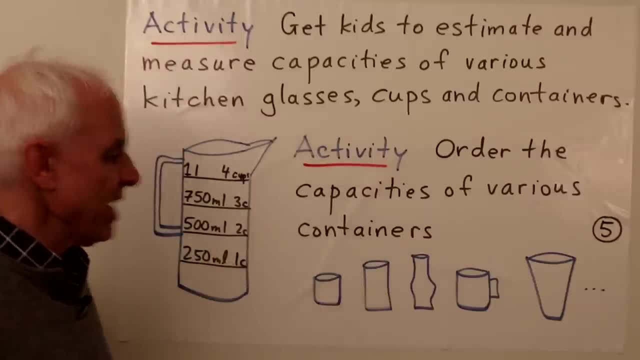 kind of fun and this gives kids experience again connecting the abstract numerical system with something that's tangible, that's physical, that they can get. So it's a very direct kind of thing. Pouring water from one thing to another is kind of fun and this gives kids experience again connecting the abstract numerical system with something that's tangible, that's physical, that they can get. 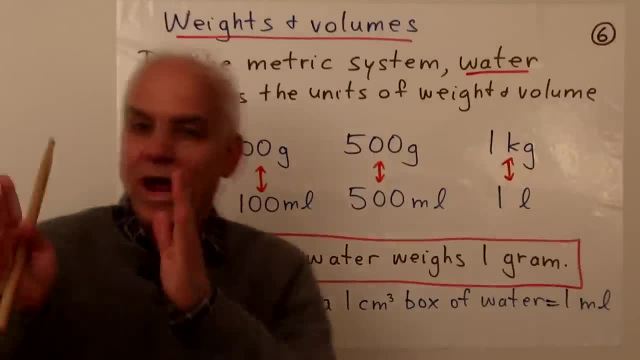 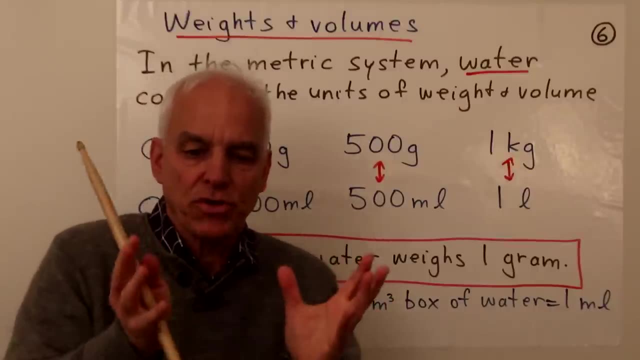 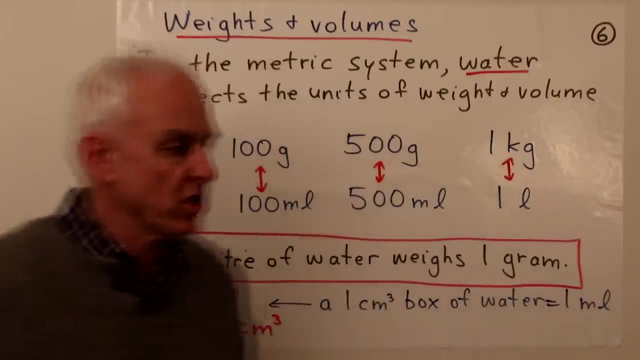 their hands on. so these two measurement systems of weight and volume are closely connected, and sometimes it's reasonable to measure the quantity of something either by a weight measurement or volume measurement. both of them give us interesting information, And in the metrical system the two scales that we're using are naturally linked, and they're linked by. 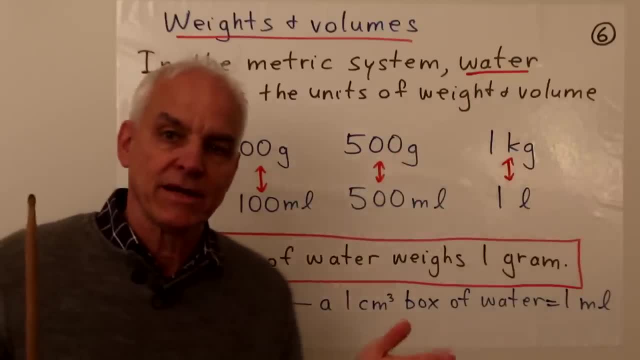 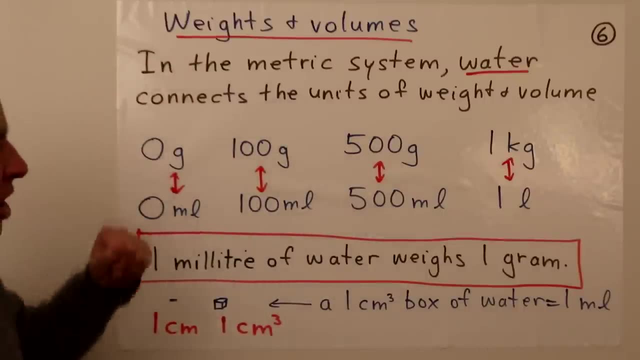 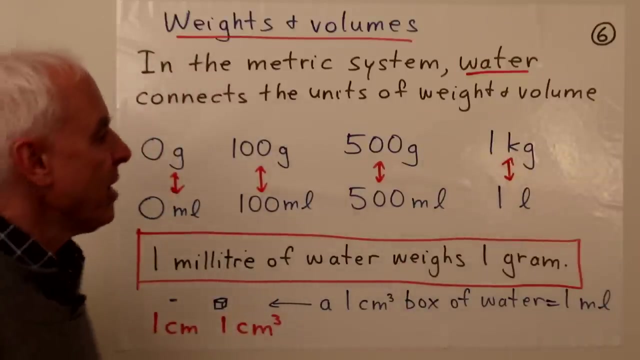 water. So water is the connection between weight and volume, between the units of weight and the units of volume in the metric system and the way that works. we've already talked about this- that the definition of one kilogram, well up to relatively recently, was that it's the weight of water. 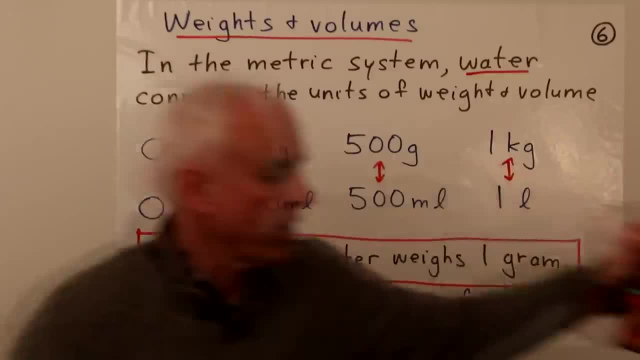 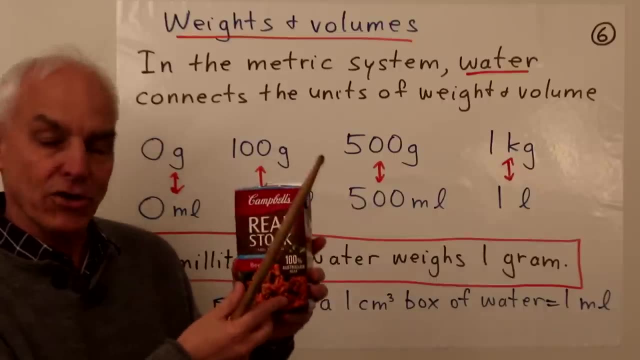 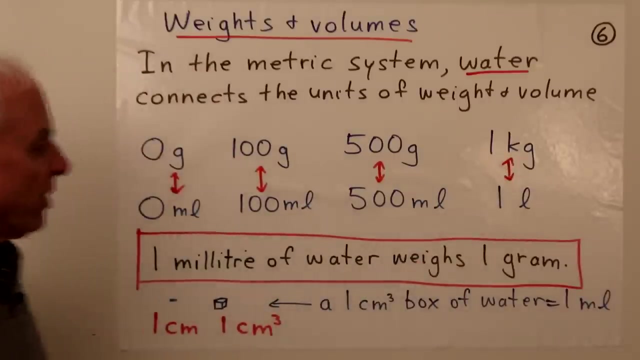 contained in one liter. so if this was water instead of beef stock, then the weight of this one liter of water would be one kilogram. okay, so one kilogram corresponds to one liter, and since the kilogram is divided into a thousand grams and the liter is also divided into a thousand milliliters, there is then a 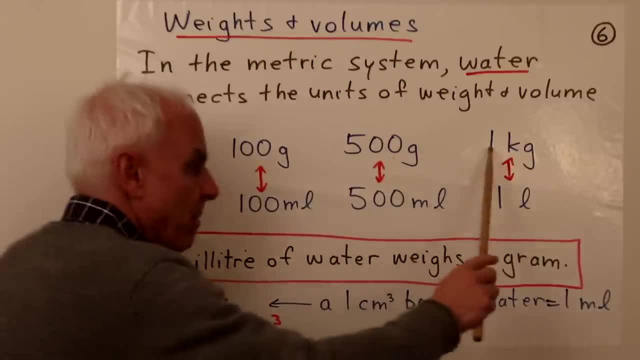 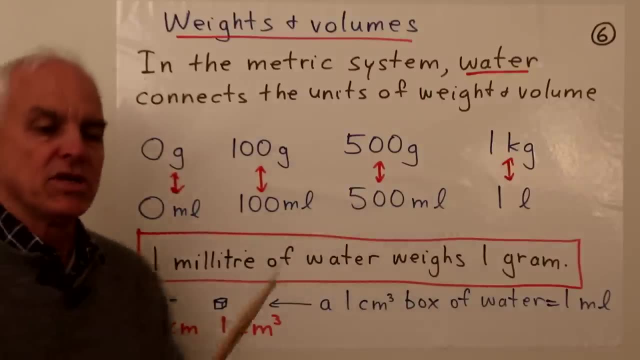 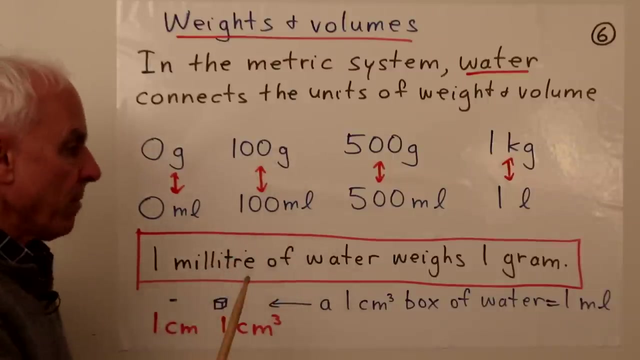 precise correspondence between the number of grams that a certain amount of water wastes and the amount of milliliters which is its capacity. so a hundred milliliters of water will weigh a hundred grams, 500 milliliters of water will weigh 500 grams, and so on. so that's a very simple. 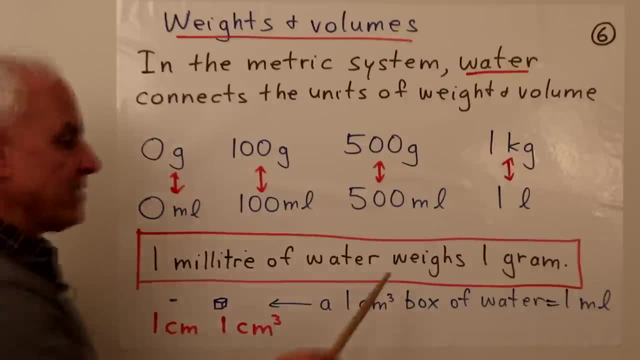 system and, of course, one milliliter of water weighs one gram. and how much is a milliliter of water actually in terms of sort of a volume? well, it turns out to be just a cubic centimeter. okay, so a centimeter is about this. it's a little. 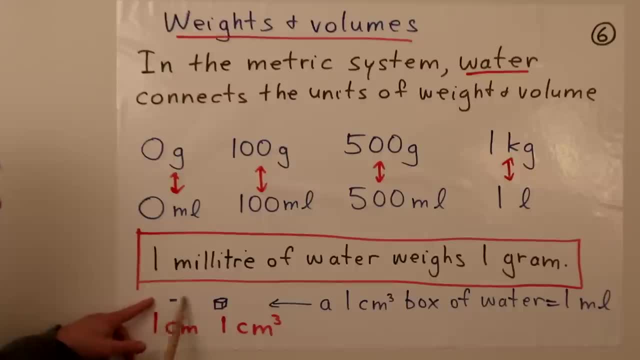 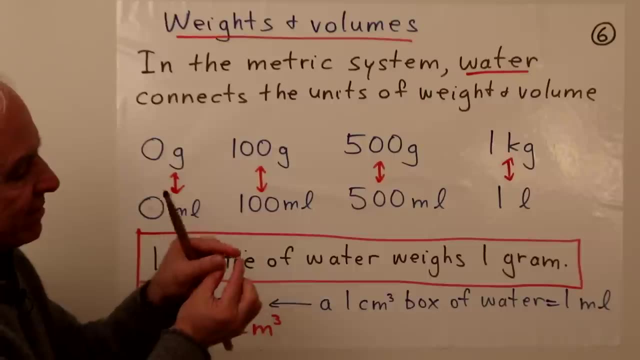 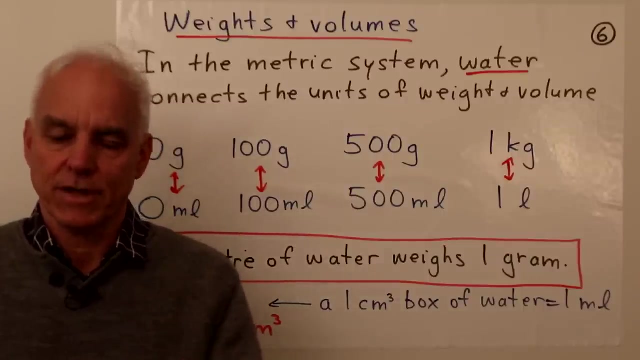 bit less than half of an inch. there is a centimeter, okay, and here is a little box whose sides are all 1 centimeters, so it's a very little box, okay, and that volume is 1 milliliter, okay, and so that volume of 1 milliliter. 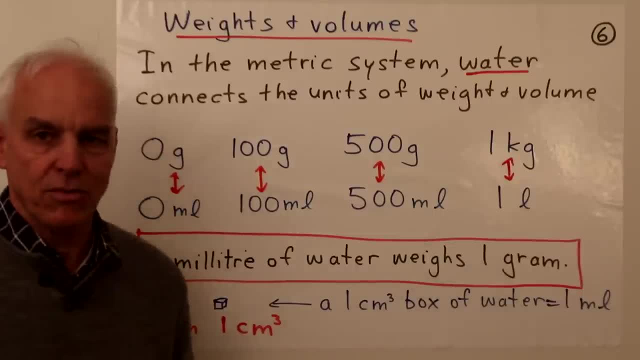 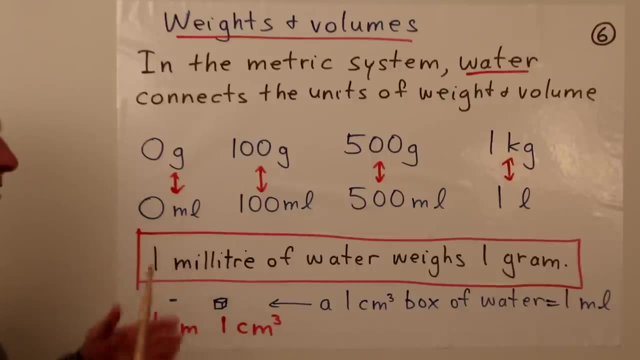 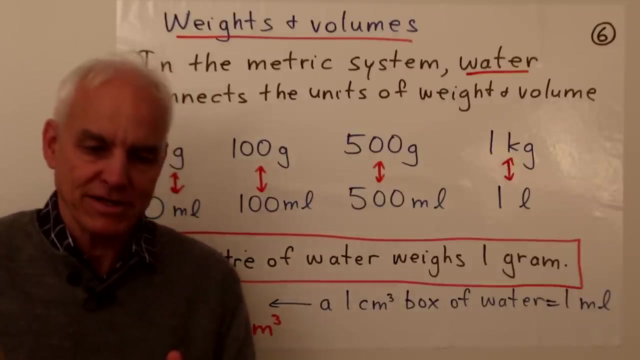 is 1.0섬 would weigh one gram if it was filled with just water. So in the metric system everything works quite nicely with respect to water. But we might say we might mention that if you have some other substance not water, maybe vinegar or 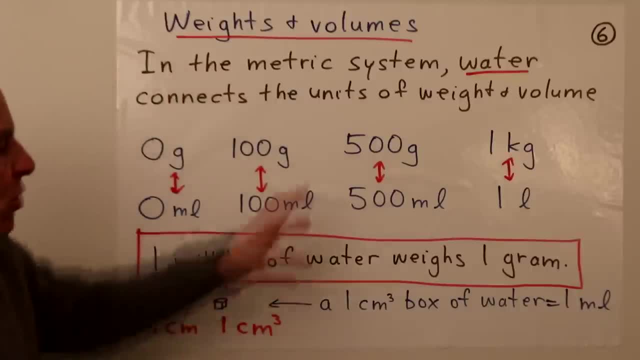 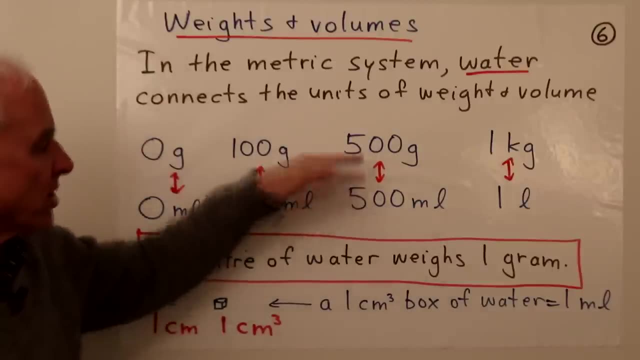 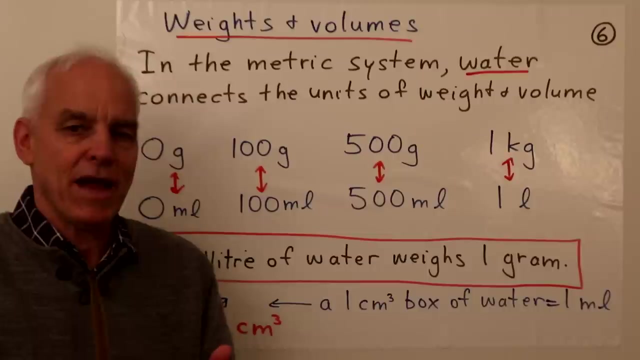 maybe beef stock or something else, then this correspondence between weight and volume is going to be different. There's also going to be a correspondence, but it's going to be more subtle and it depends on the nature of the substance that you're talking about. So that brings us to the topic of density, which is: 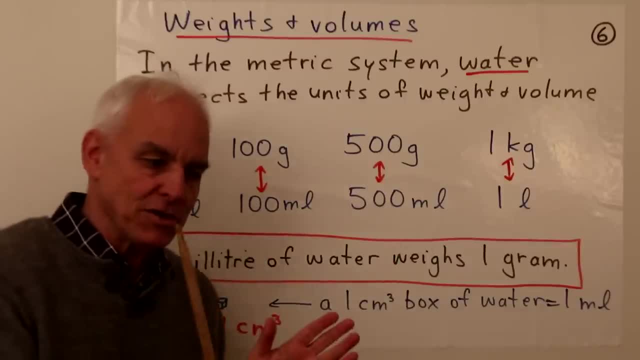 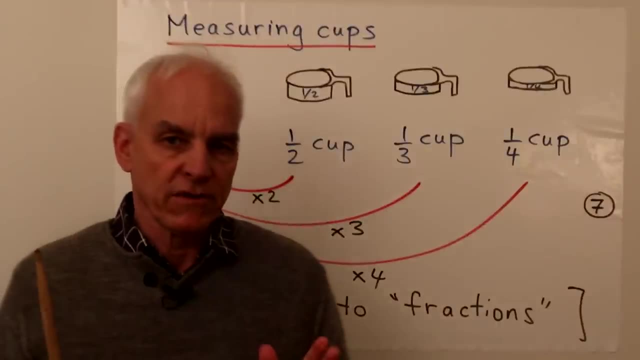 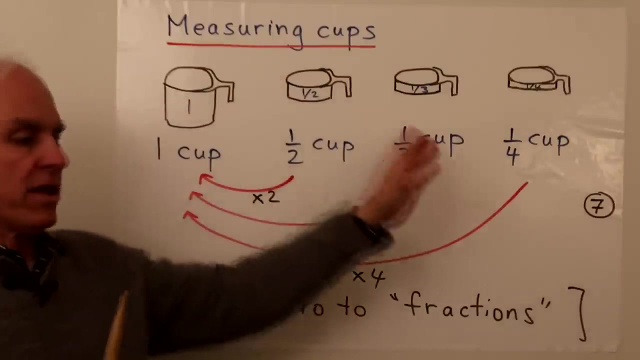 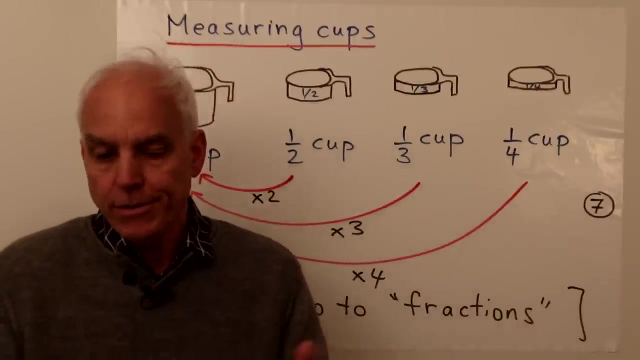 something that we can learn about later on, once we've mastered weights and capacities. So especially useful for young children, who perhaps want to help out in the kitchen to understand that there are these measuring cups that help us in understanding volumes and capacities of fluids or other things like grain or 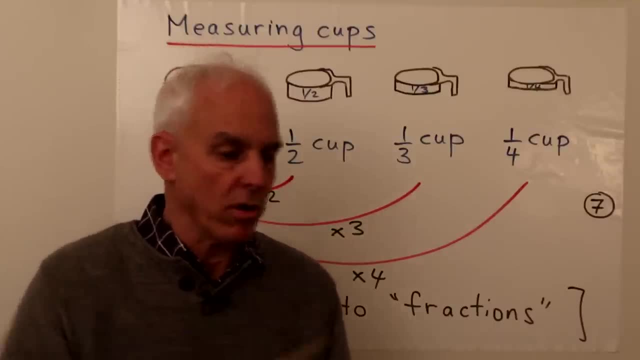 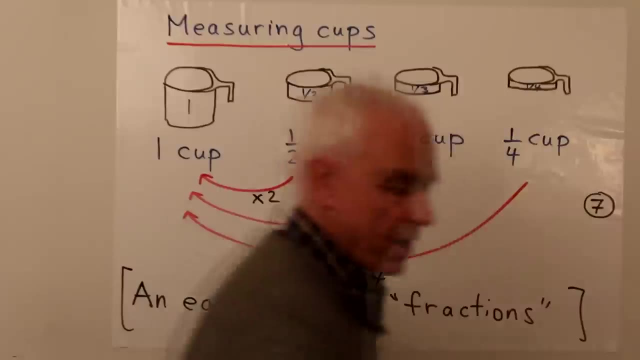 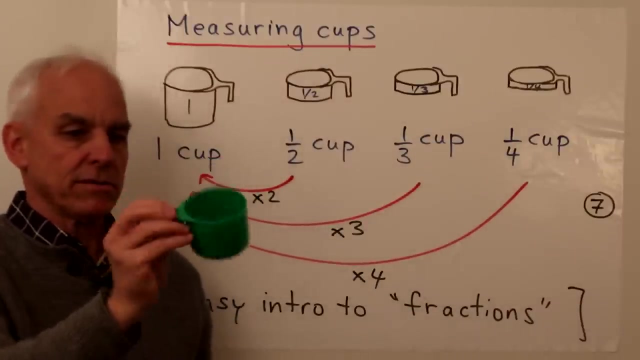 sand, even anything that pours. So here's sort of a standard system of cups, a one cup unit- I've got some here, so it's just borrowed from our kitchen. There is a one cup unit, A unit. It says one cup on it. There it is there, And then next smaller unit is a. 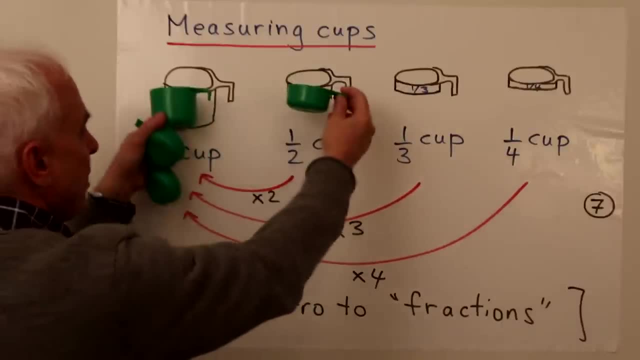 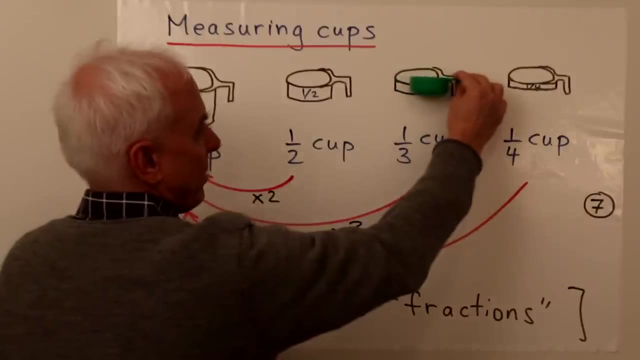 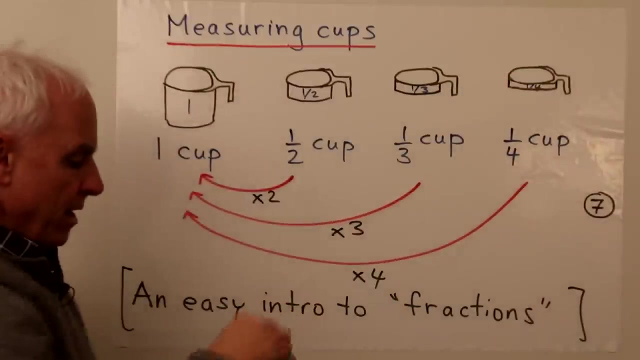 half a cup And there's a half a cup, There's one cup, There's a half a cup, And then a third of a cup, A third of a cup And finally a quarter of a cup. Okay, And these have little indicators on here which you might not be able to read, but 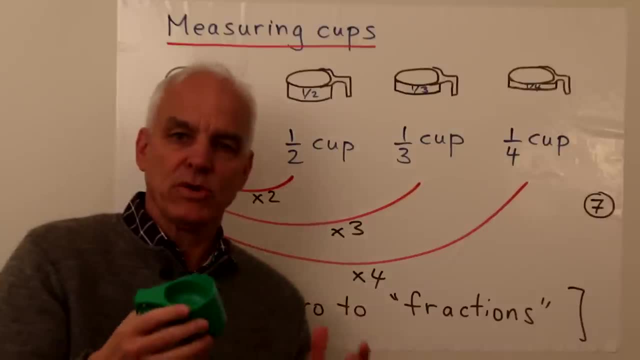 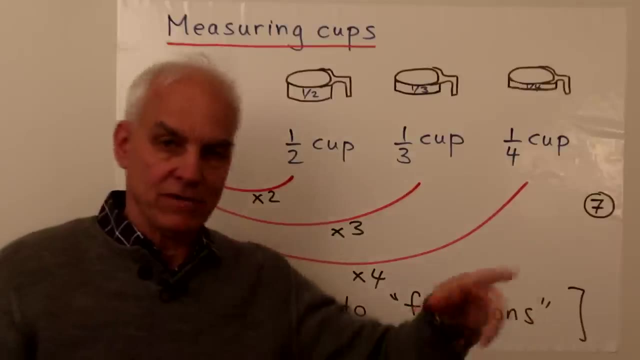 anyway, This kind of system of measuring cups. it's also a very useful thing to have in a classroom. Okay, Ideally, actually, classrooms should have little water sinks, Places where you can pour water And fiddle around with water and volumes and so on. 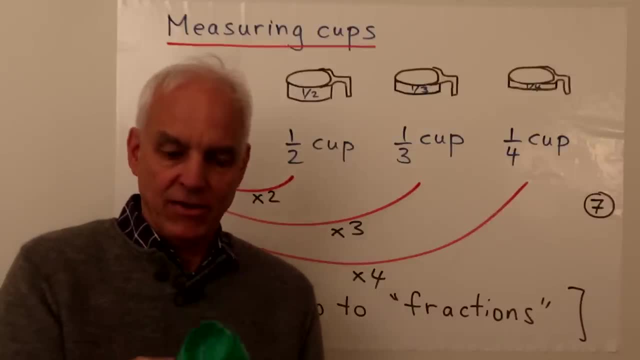 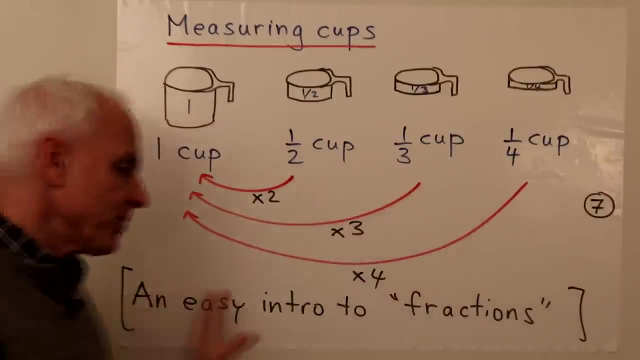 That's very handy thing to have And something like this is a great tool to help kids start to appreciate not just volumes, but also we're touching base, as you can see, with the idea of a fractions. So we are talking about fractions, but don't use the word fraction. don't tell kids that. 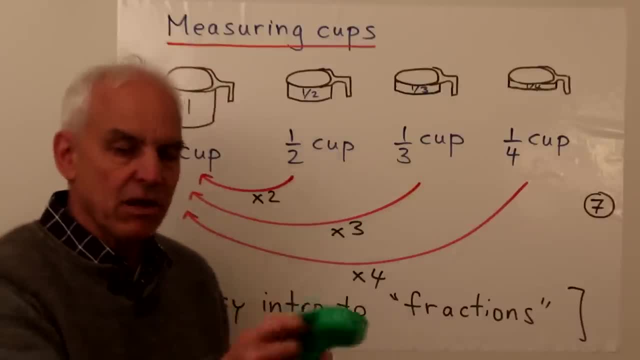 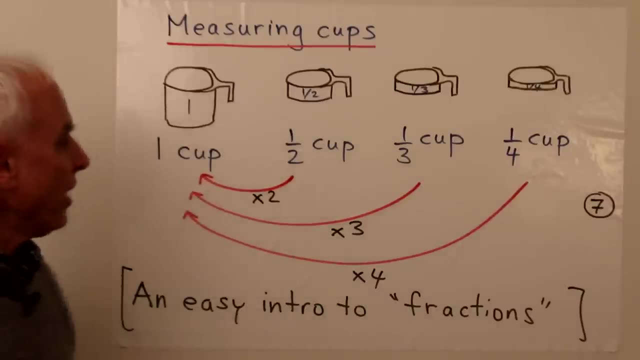 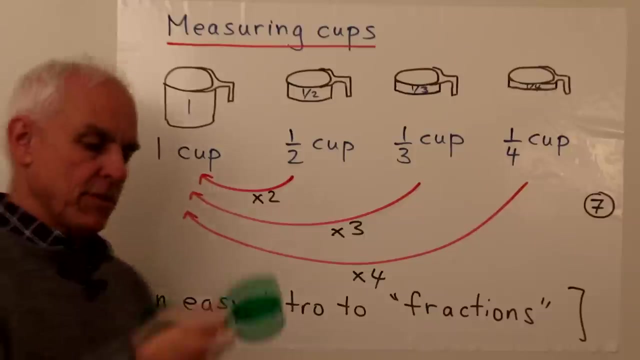 okay, now we're doing fractions. We're not doing that. We're just using these very particular measuring cups to help us measure stuff, And all what they need to know is that two of these half cups equal one cup. Two of these make one of these, and they can test that by filling this with water twice. 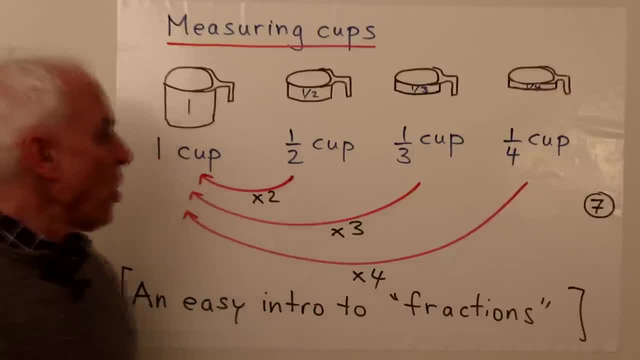 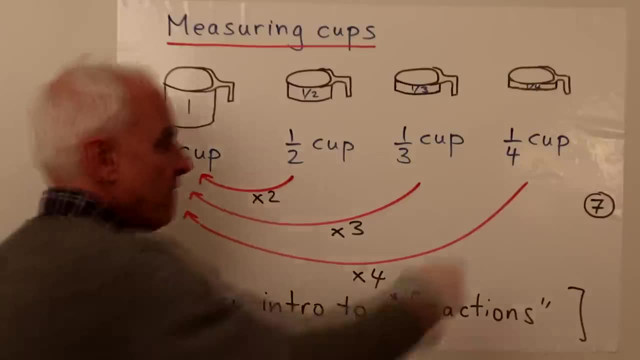 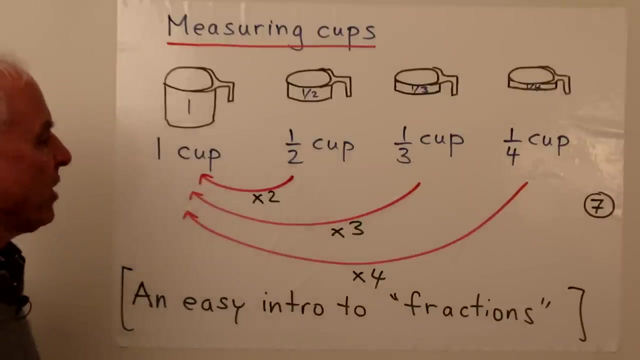 and you'll get right up to the top of that second one. And similarly, three of these one third cups give you the big one, And similarly, four of these quarter cups give us a cup. So that's the crucial property of these smaller subdivisions. 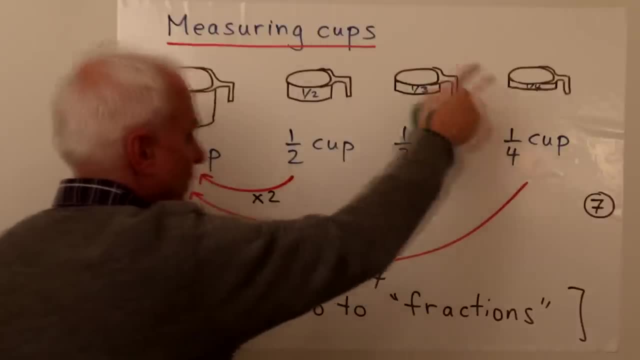 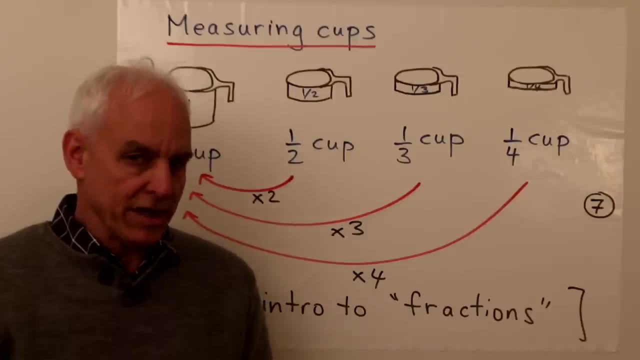 Two of these is a cup, three of these is a cup. four of these is a cup. So we're learning a little bit about fractions. just a very brief introduction in the context of measuring, and there's lots now of stuff that children can do. 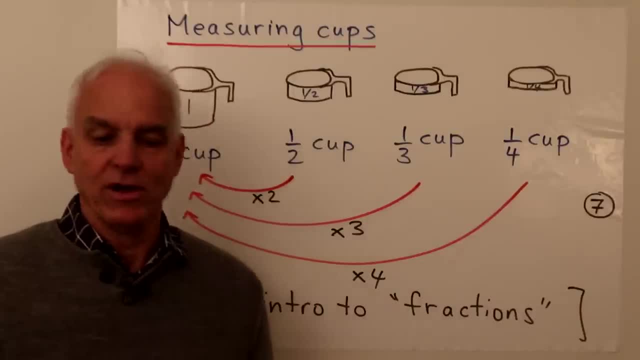 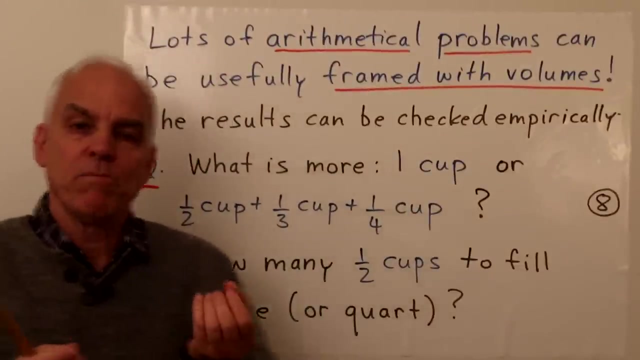 Lots of investigations to make, lots of questions that one can pose, lots of little problems to solve, little fun activities to do because we're pouring around with water and stuff and it's all kind of fun. Now there's a lot of arithmetical problems now that can be posed in terms 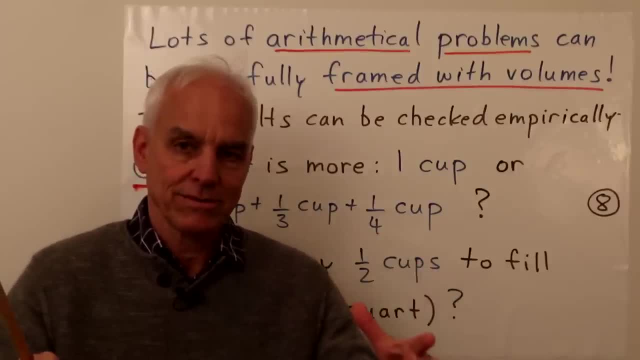 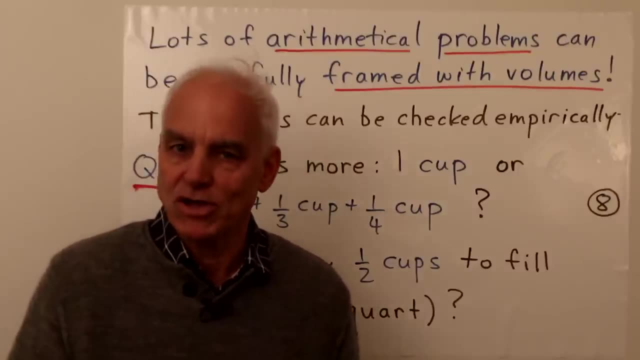 of this framework of volume measurement. So that gives some meaning to otherwise perhaps unmotivated arithmetical questions. And in the course that I'm going to put together here, I'm going to give you lots of examples in this direction. So easy questions, not so easy questions, some challenging ones for students to get. 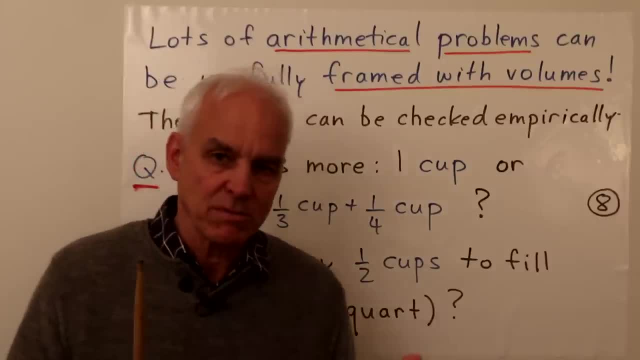 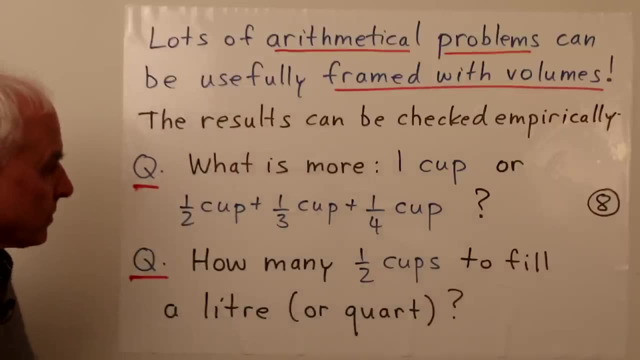 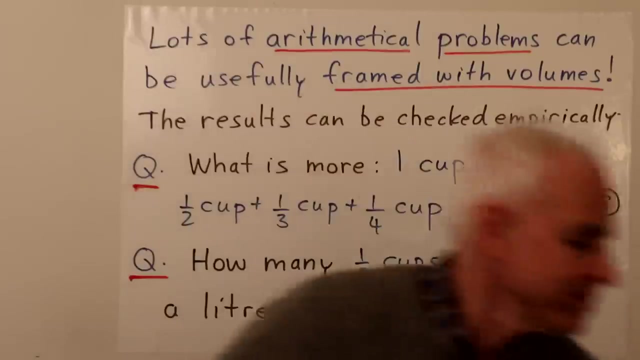 experience doing arithmetic in the context of something very special, Something very specific: in the context of weighing and measuring volumes. So, for example, what is more One cup, or one half a cup, plus one third a cup, plus one quarter of a cup. Okay, so, going back to our measuring ones, there's the one cup and there are the other. 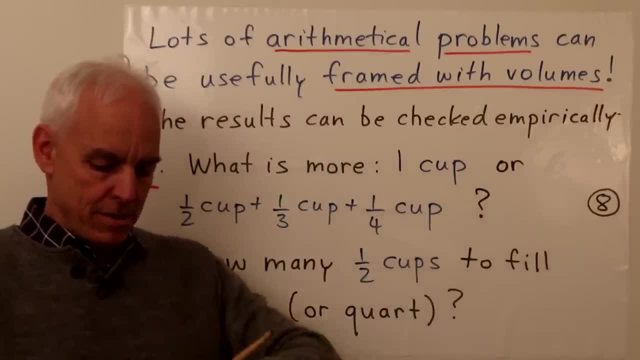 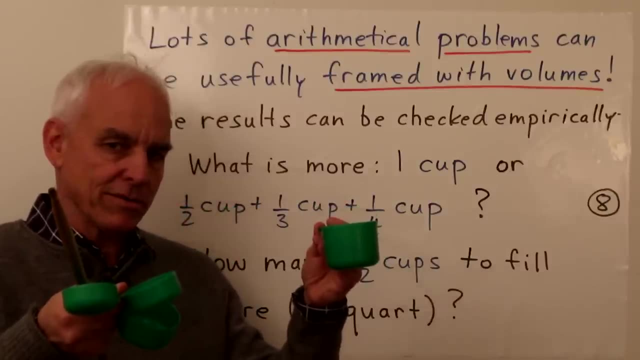 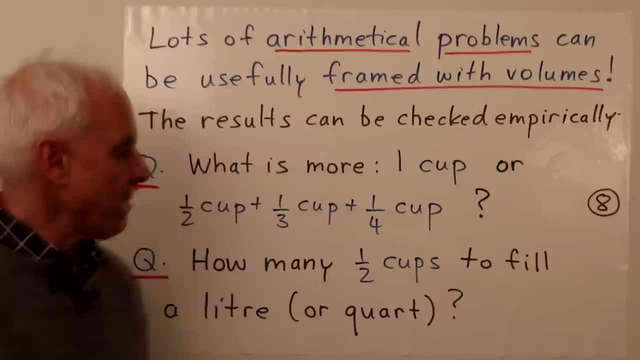 three, And if we fill all these up, we fill this one up, Which one has the most water. Okay, so that's not that hard, but it's not that easy either, and some understanding has to be brought to bear here, right? 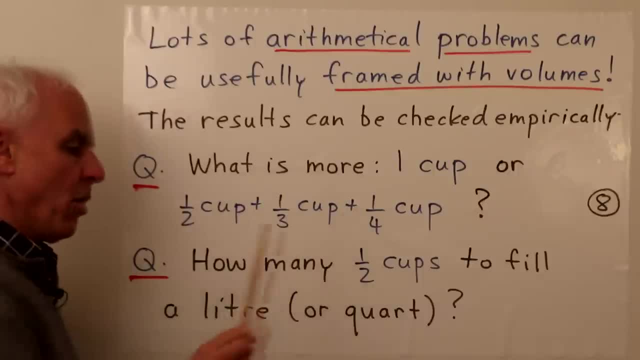 They have to have some sense of what the meanings of these things are, and all what they need to know is that two of these make a cup, three of these make a cup and four of these make a cup. Another kind of question is how many say half a cups will be required to fill a liter.